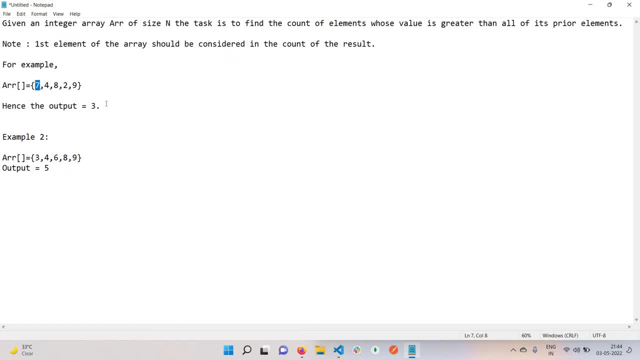 So hence, we have 3 elements like this, Like 7,, 8 and 9.. So the output will be 3.. And same, in this example, Every element is greater than the prior elements, Like, if we take an example of 9.. 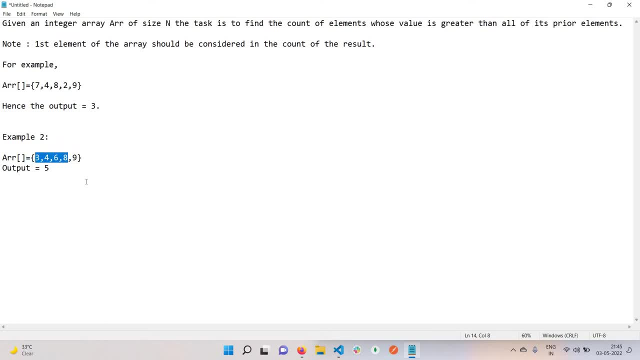 These all elements are less than 9.. And if we see the example of 8., So these are less than 8.. Like this, So the output will be 5.. So yeah, let's go to this question. This is quite an easy question. 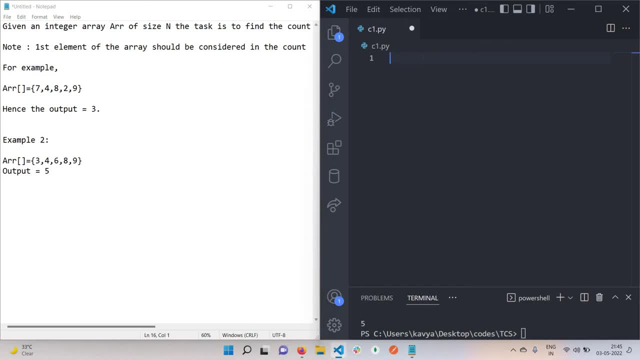 So the input will be The first line will have the number of elements inside an array. So we can simply- I am using Python, You can use any one. So this is- I am just taking the input. This is the number. 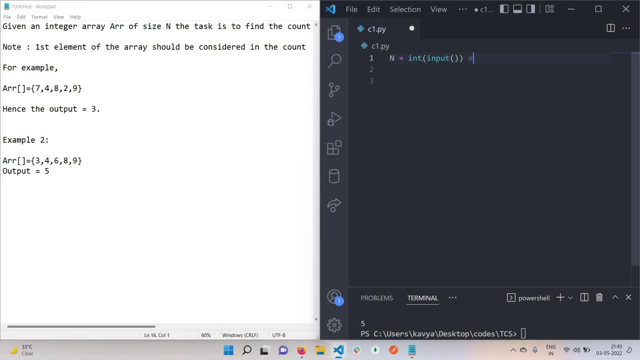 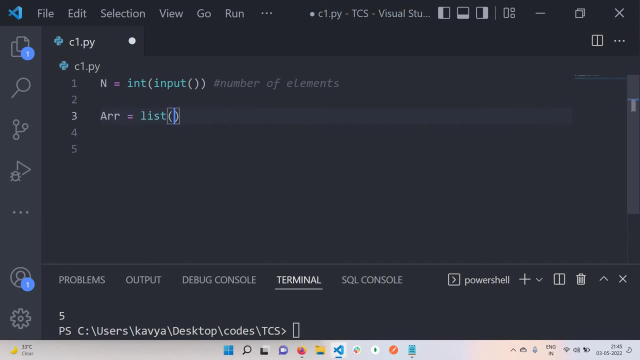 Basically, it represents the number of elements in an array. So elements. Let me increase the font, Okay. Increase the font, Okay. And after that this is an array, So I am using the list map, So this is one of the best methods to take space-separated values. 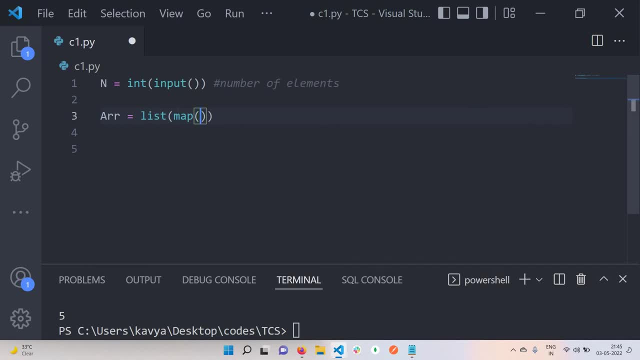 If you want to use a Basically line-wise value, So you can simply trade using for loop, List, map, End, Input, Split And the count of the number is like this: Okay, So it will. It will give our array, which has some values. 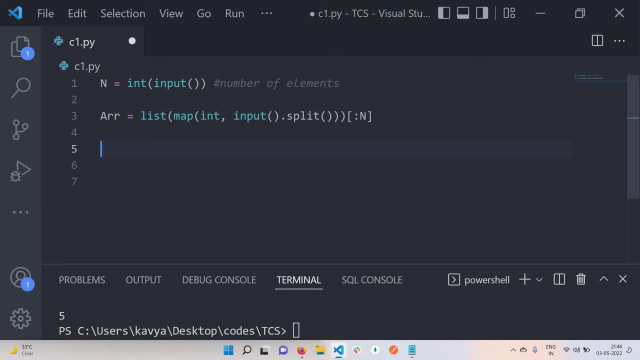 We will print. And the next thing is I am just taking two variables. One is targeting the max value Initially assigned to 0. And the second is, like our answer count, It is also 0. So it will target the maximum value. 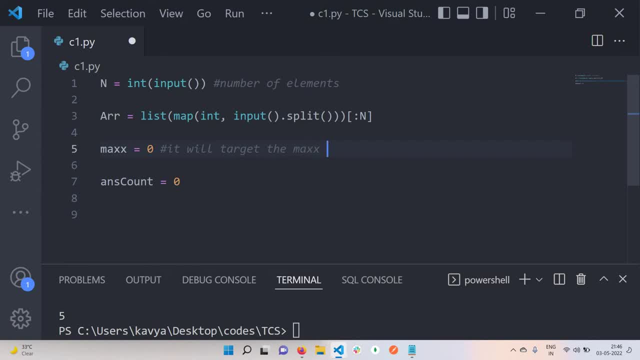 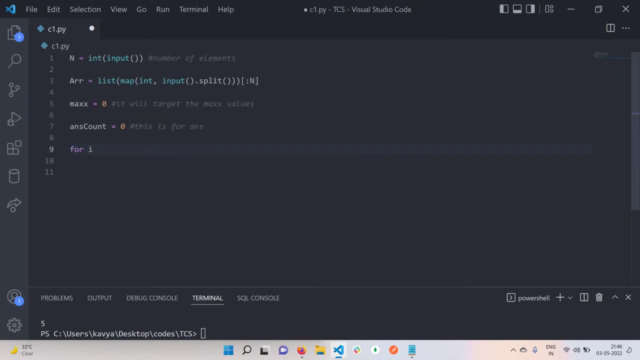 It will Target the max value. This And this is answer. This is our answer. Okay, And now just iterate over this array. for i in this array And if we counter any i which is greater than max value, See: 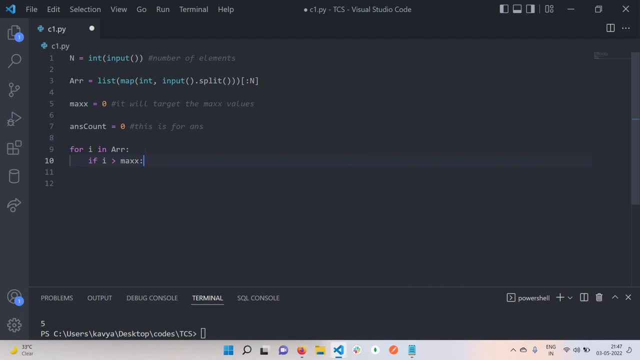 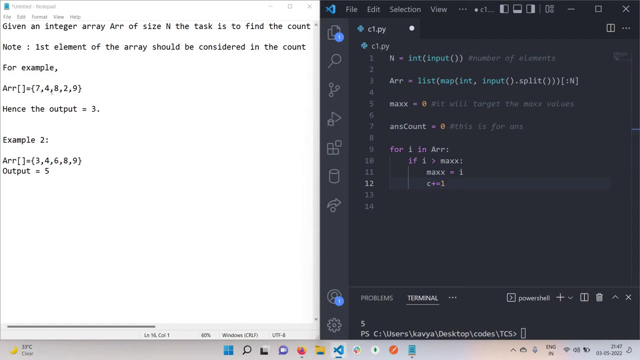 If we counter any i which is greater than max value, So our max will be that i, and also we got our first element because we are traversing array through the left side. suppose we have values like like a, 7, 4, 8, 2, 9, and the first 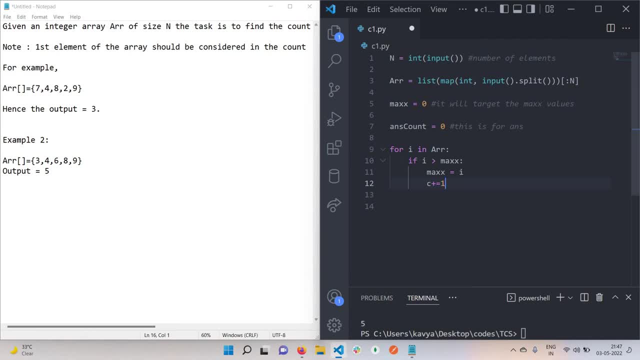 value will be 7, so 7 is greater than I. max is basically 0. so you have: 7 is greater than 0, so max will be 7 and our count is also increased. next value we will get is 4, but here, you see, 4 is greater than max. it is not so just. 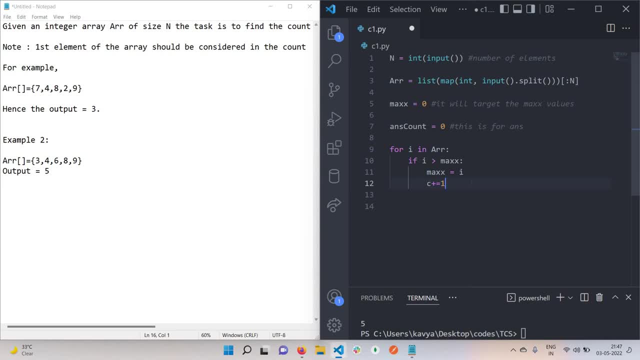 neglect this and things and things will come okay. so like this: yeah, this is just a code. just print this counter value, not a C. basically, we have answer count as our answer, so just print this count value and you will get the answer. okay, so this is the code. 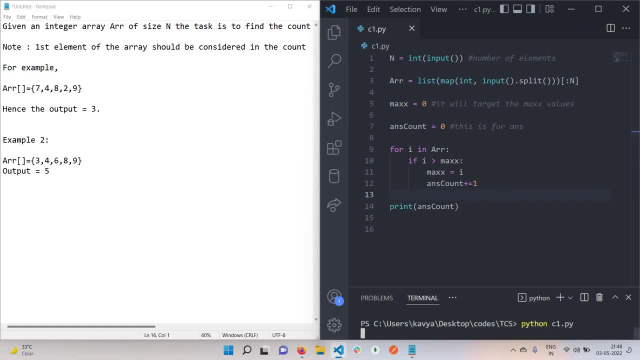 that we need to write. okay, suppose the total number of element in first array is 5 and the element that we need is like a 7, 4, 8, 2, 9, so the output will be 3. okay, we got this. and the next input we have like 5 is the size, and like a 3, 4, 6, 8, 9, so our output is 5. we can also check for the random inputs like: 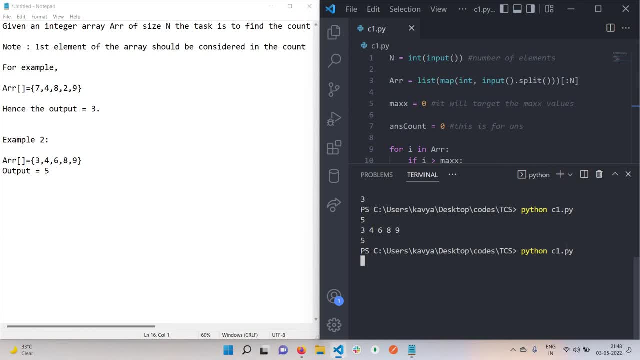 we can also check for the random inputs, like. we can also check for the random inputs like: suppose and using making said against id8 and the values. I am putting like 14. and suppose and using making said against id8 and the values. I am putting like 14. 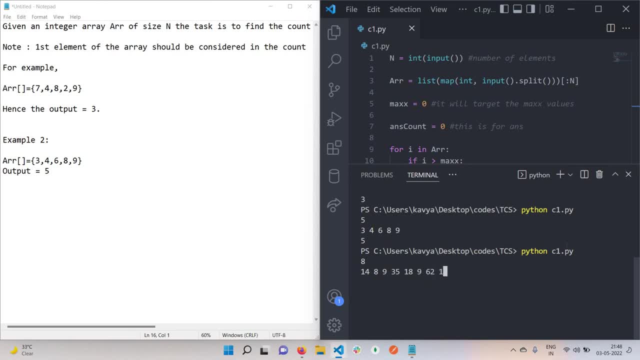 628932. we got on set 3 because first element always included in our answer: the count. we got on set 3 because first element always included in our answer. the count is 1 now and if we see 35, all the values on the left side of 35 is less than 35, so one. 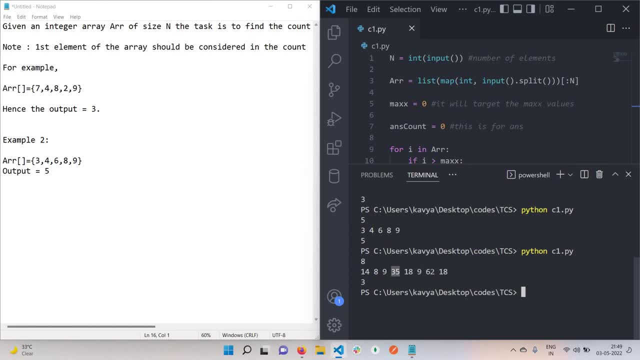 person, that is 2 and 19. this is not true. yeah, for the 62 we have, all the values on the left is less than 62, so this is also included. our answer, so our output is like a 3. so, yeah, this code is working for all test cases. so this is.